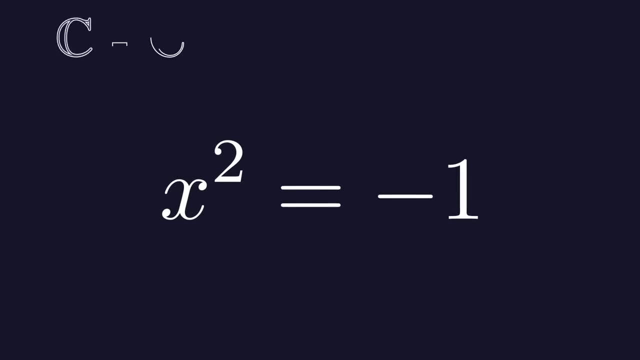 number that, when squared, gives a negative result. This is where the complex numbers come in. We define i as the number which, when squared, equals minus one. With i we can find square roots of other negative numbers. For example, the square root of minus nine is 3i, because 3i squared. 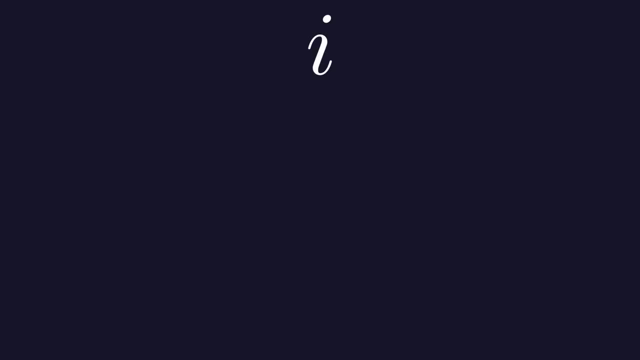 is equal to minus nine. When we multiply i by itself repeatedly, it creates a cyclic pattern: i minus one, minus i, one and again i. To understand Euler's identity and the number e, we first need to know about derivatives. The derivative describes the rate of change of a. 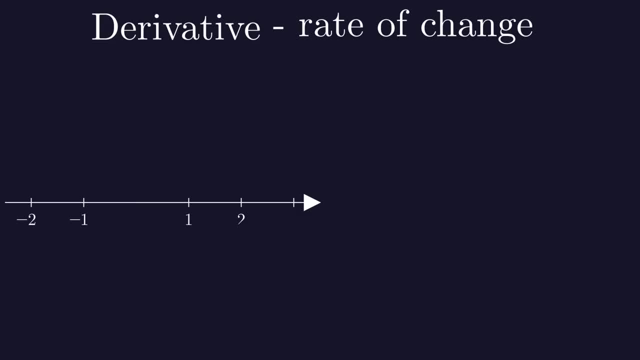 function at any given point. Let's look at a graph of a function: x cubed minus two, x squared minus three, x plus three At x equal to minus two. this function is x squared minus two, x squared and minus function increases rapidly, but as x approaches about minus 0.4, the increase slows down. 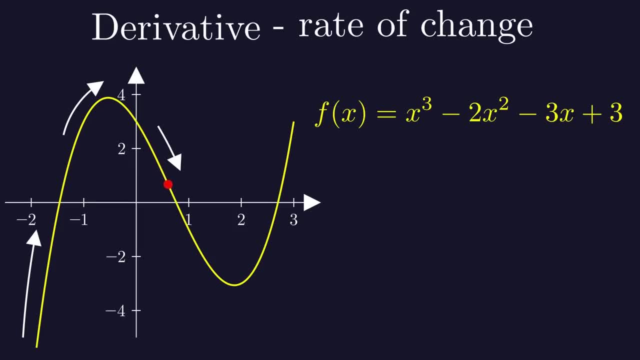 the growth rate goes to zero and after this point the function starts to decrease. That's what a derivative measures. The value of the derivative at any point is also equal to the slope of the line tangent to the graph of the function. at that point, The derivative 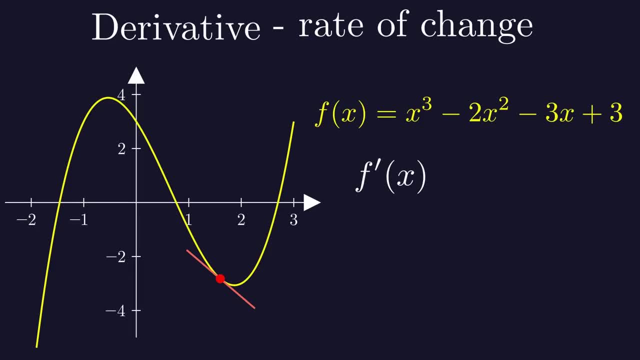 of the function f is denoted as f prime or as d over dx. To calculate the derivative, let's start with calculating the slope of the line going through two points. Suppose we pick two points on the graph at x equal to a and x equal. 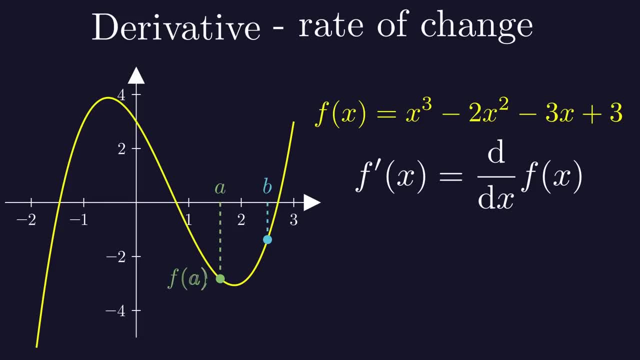 to b. Their y coordinates are respectively f and f, so the height difference between those two points is equal to f minus f. The horizontal distance between these points is equal to b minus a. Let's call that length h. Now we also can write f as. 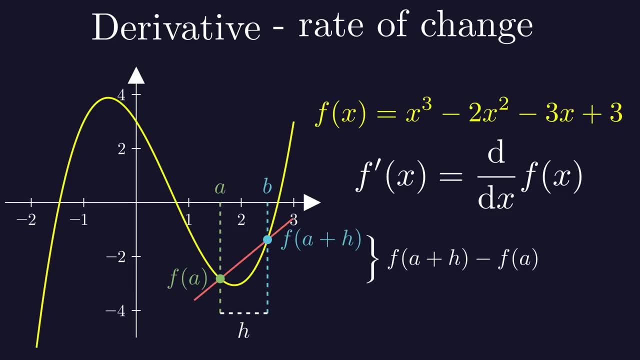 f. The slope of the line going through those two points is equal to f plus h minus f divided by h. This formula would give us the average rate of change between points A and B, But a derivative describes the rate of change at a single. 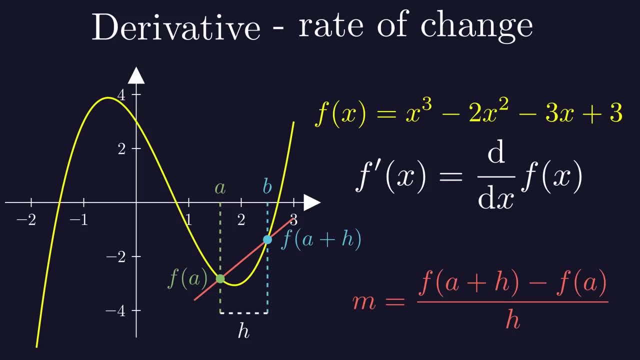 point, not over an interval. So to calculate the slope of the tangent line at point A, we just have to make h very small, As h gets closer and closer to 0, B gets closer and closer to A. So to calculate the slope of a tangent line at 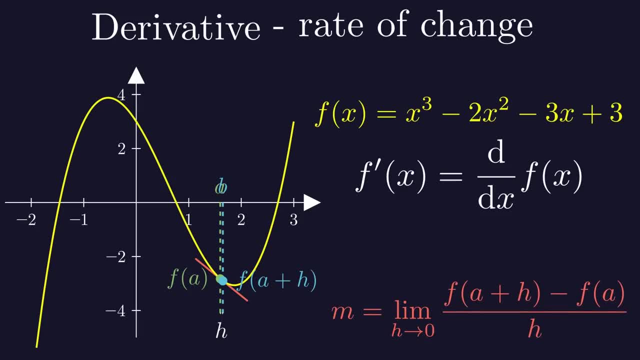 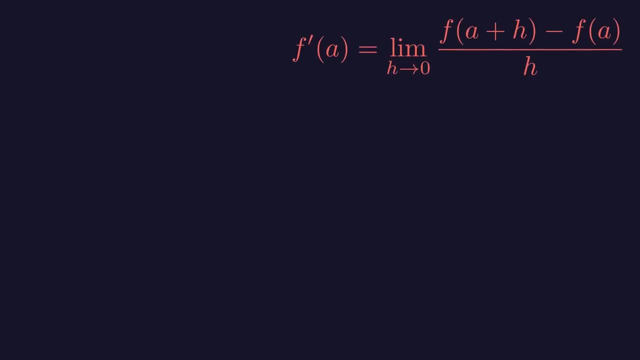 point A. we just have to take a limit as h approaches 0.. And exactly that is the definition of the derivative. To see how it works, let's look at a simpler function. For example, f of x equals x squared. Let's calculate the derivative. 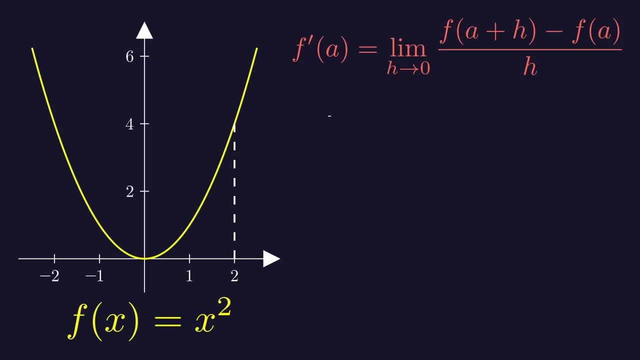 of this function at point A equal to 2.. From the definition of a derivative f prime of 2 is the limit, as h approaches 0, of f of 2 plus h minus f of 2. divided by h, That is equal to the limit of 4 plus 4h. 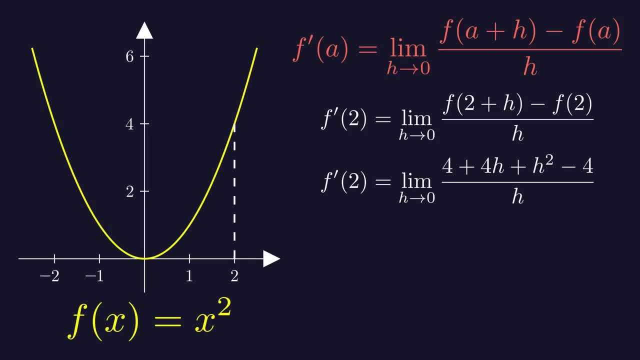 divided by h, That is equal to the limit of 4 plus 4h. divided by h, That is equal to the limit of 4 plus 4h plus h squared minus 4. divided by h, And after simplifying, that is equal to 4. 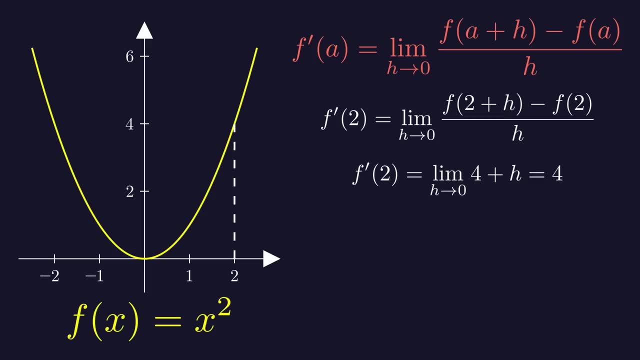 plus h, As h approaches 0, this is just equal to 4.. So the value of the derivative at A equal to 2 is 4.. But we can find a general formula for the derivative of this function. To do this, we calculate the f prime of x instead of. 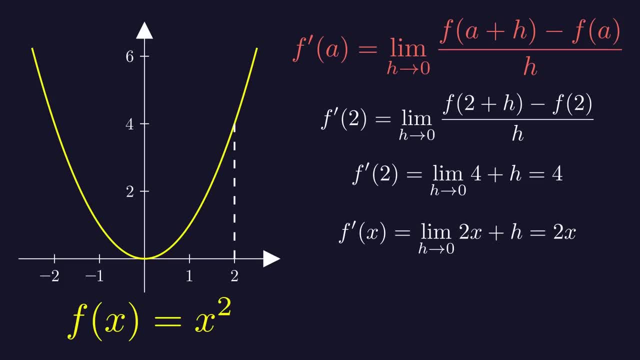 2. After simplifying we get that f prime is just equal to 2x. So the derivative of f of x equals x squared. at any point, x is just equal to 2x. Calculating derivatives doesn't always require using the definition. There are some. 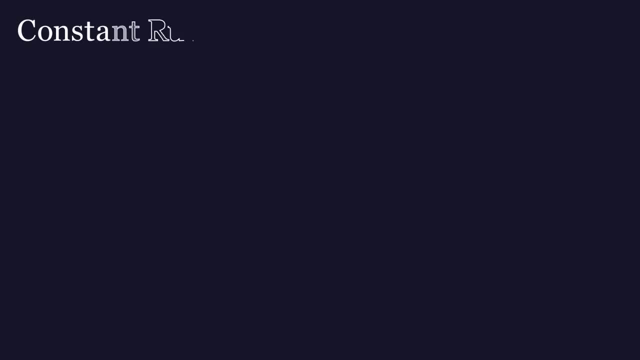 rules and shortcuts that can make it easier. The constant rule tells us that the derivative of a function multiplied by a constant is equal to the derivative of that function multiplied by that constant. For example, the derivative of x squared is 2x, So the derivative of 3. 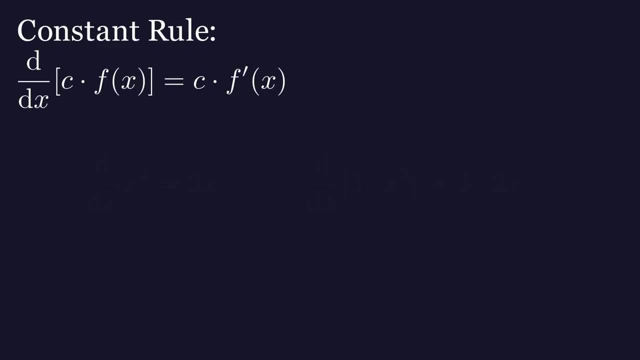 times x, squared will be equal to 3 times 2x. The sum rule tells us that the derivative of a function that is a sum of functions f and g is the sum of the derivatives of those functions. The last rule that we will need to understand Euler's identity is the power rule. This: 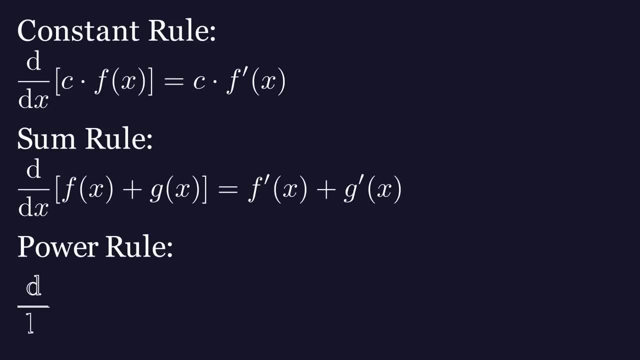 rule tells us that if we have a function that is of form x to the power of a, the derivative of this function is equal to a times x to the power of a minus 1.. For example, the derivative of x to the power of 4 is equal to 4 times x cubed. 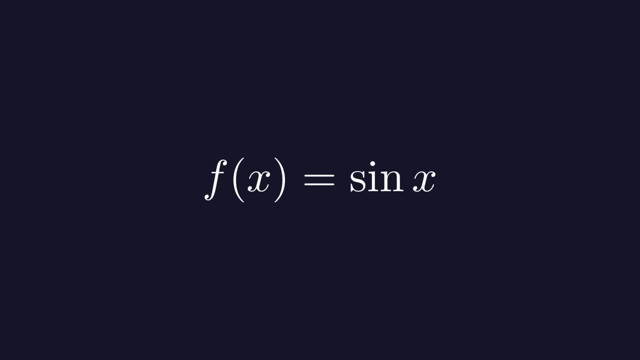 Finding derivatives for some functions like sine of x requires a bit more work than just using those rules. We have to go back to the definition of a derivative. From the definition, the derivative of sine of x is the limit as h approaches 0 of sine of x plus h minus sine of x divided. 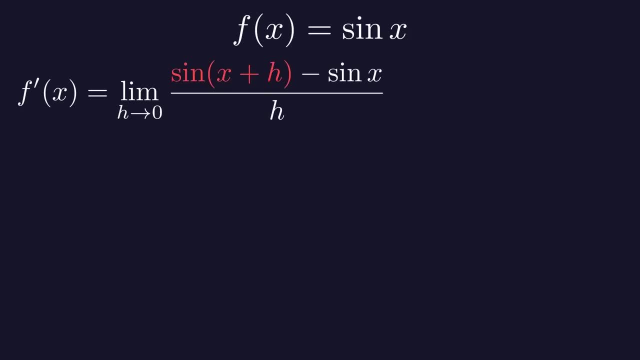 by h. We can use a trigonometric identity to expand sine of x plus h into sine of x times cosine of h plus cosine of x times sine of h. Then we divide this expression into two parts. From the first fraction we can factor out sine of x. From the second fraction, we can: 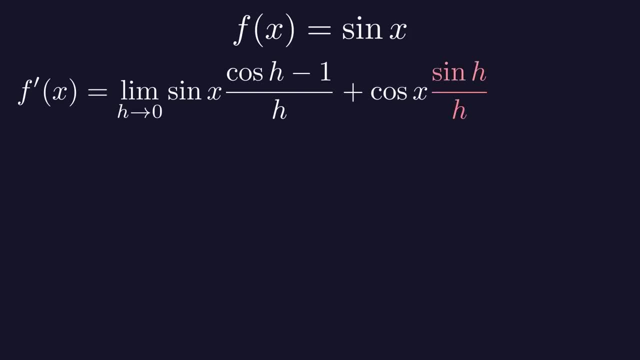 factor out cosine of x. Let's first see what happens to the sine of h over h as h approaches 0.. Imagine a circle with a radius of 1 and an angle of h radians. The length of the arc created by this angle is also h. The line perpendicular to the radius is equal to the sine of h As h gets smaller. 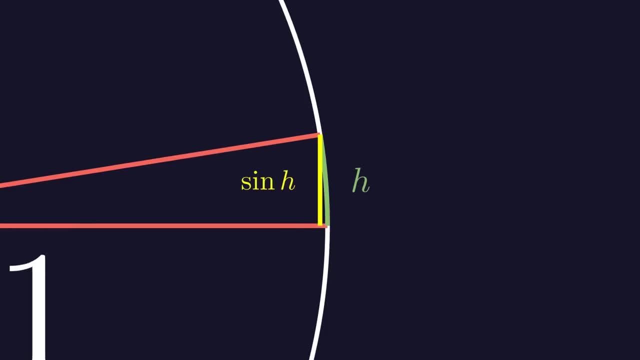 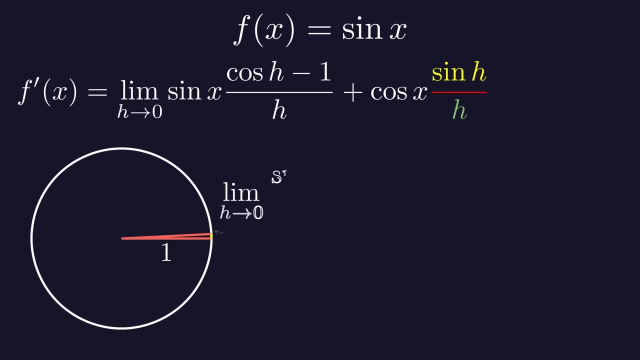 and smaller, the sine of h gets closer and closer to the arc. So the sine of h divided by h gets closer to 1.. So we know that the limit, as h approaches 0, of sine of h divided by h is equal to 1.. Knowing this, we can calculate the second part of the limit. 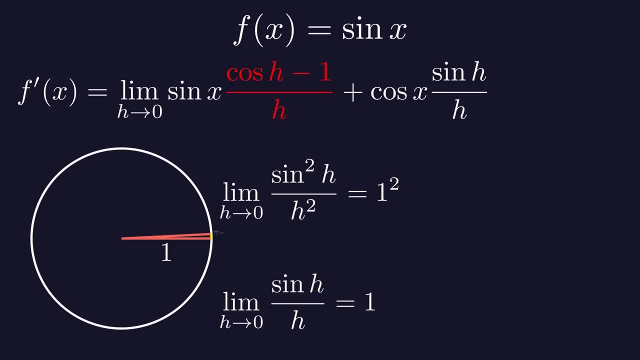 Let's square both sides. Next, we can use a trigonometric identity to write sine of h squared as 1 minus cosine of h squared. We can write it as two separate fractions and we can consider them as two separate limits. Now we divide both sides by the second limit. 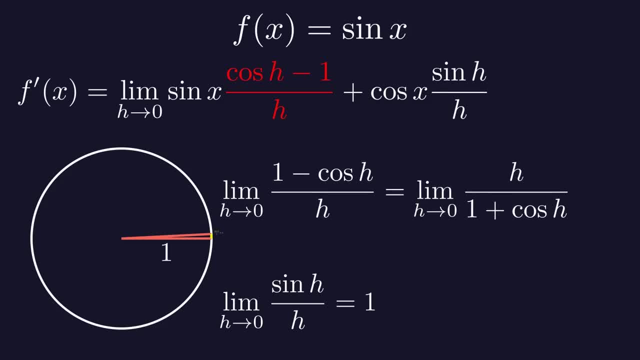 If we rearrange, the right side is equal to the limit as h approaches 0 of h divided by 1 plus cosine of h. If we add 0 for h, we find that the right side is equal to 0.. Now we multiply both sides. 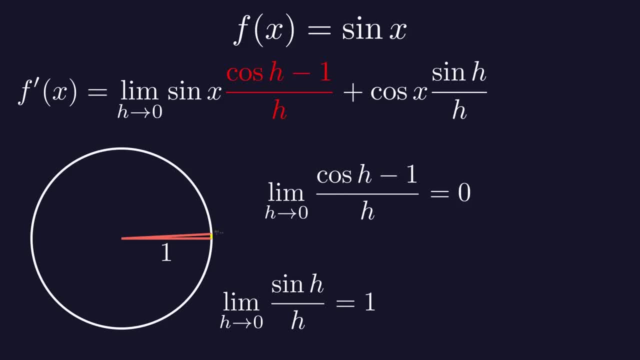 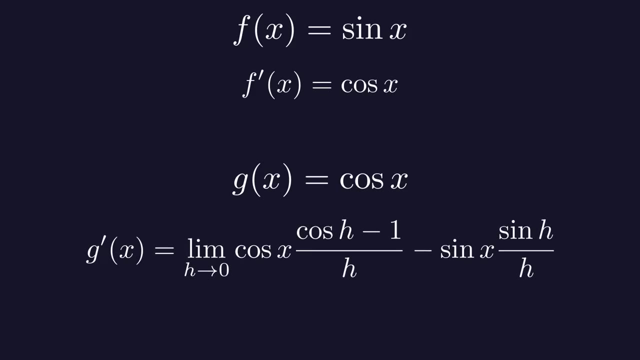 by minus 1, and we get that the limit as h approaches 0, of cosine of h minus 1 divided by h is equal to 0. So the derivative of sine of x is equal to the cosine of x. We can do the same thing for cosine, but we would get a minus sign instead of plus sign. So the 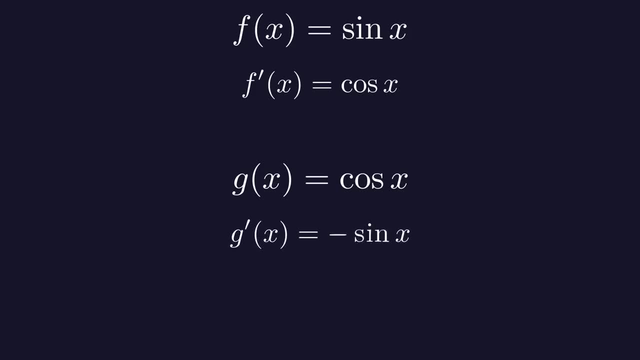 derivative of cosine of x is equal to minus sine of x. Derivatives are a very big part of calculus. If you're looking for a free and easy way to learn more about it, you can visit Brilliantorg, the sponsor of this video. 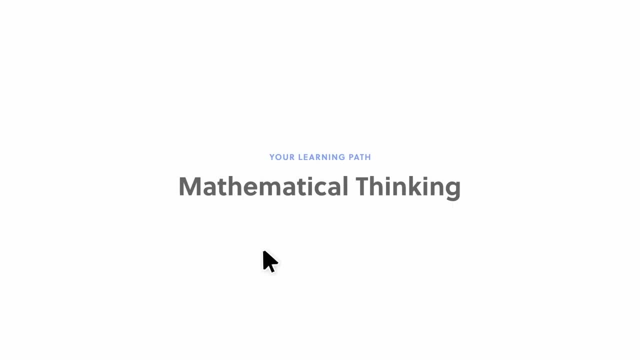 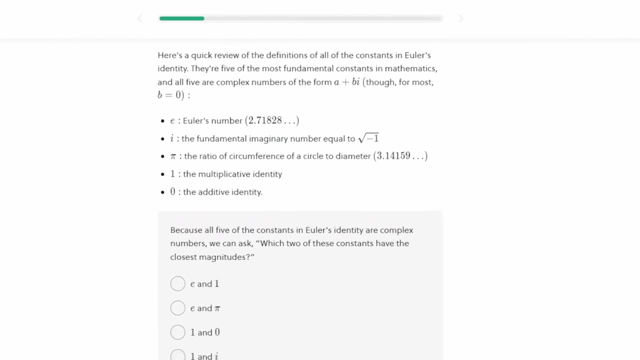 On Brilliant there are thousands of lessons on math, data science and computer science, And new lessons are added every month. In the course on complex numbers, Euler's identity is explained from a totally different perspective than in this video. What sets Brilliant apart? 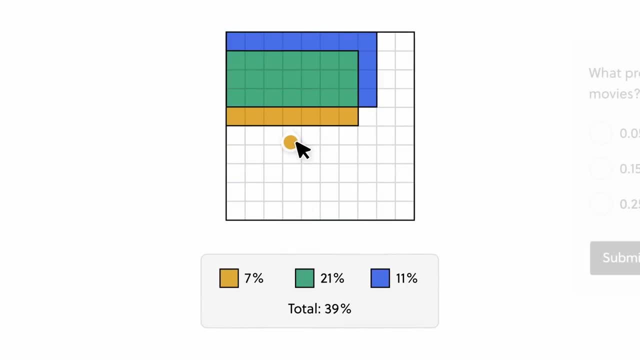 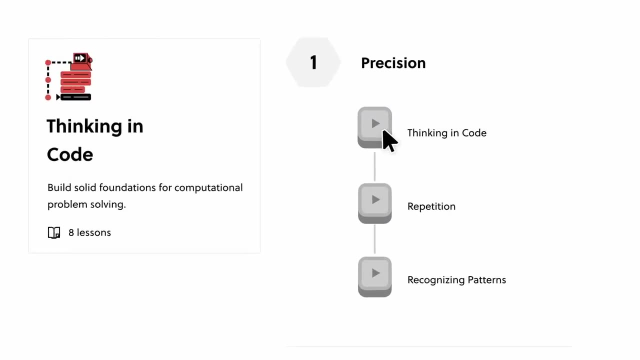 is its interactive approach. Just listening or reading isn't enough to understand complex topics. Brilliant lets you answer questions and actively engage with the content. Brilliant lets you learn at your own pace. Personally, I've been using Brilliant for over a year now. 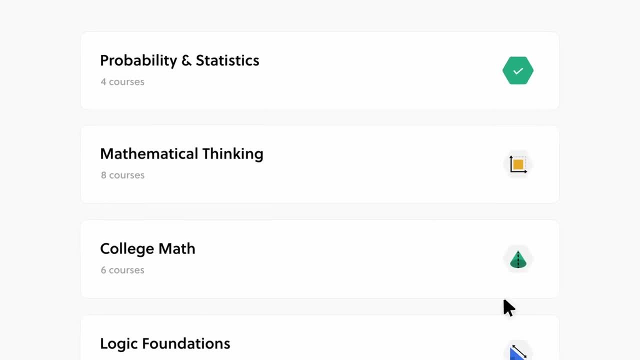 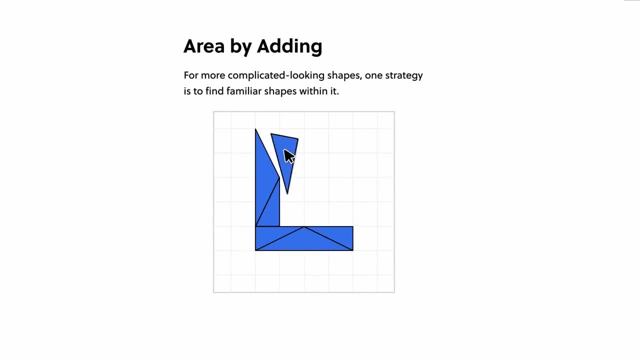 and I can say that it is the best way to learn math, data science and computer science interactively. And the best part is that you can try everything Brilliant has to offer for 30 days for free. Visit Brilliantorg, slash digitalgenius, or click the link in the description. The first 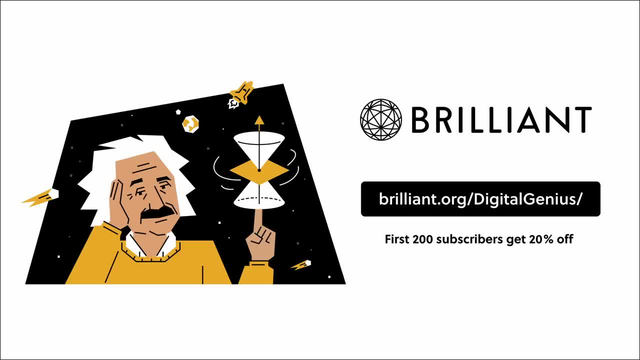 200 people will get 20% off Brilliant's annual premium service. Brilliantorg slash digitalgenius or click the link in the description. The first 200 people will get 20% off Brilliant's annual premium service. Brilliant will get a 30% off Brilliant's annual premium service. 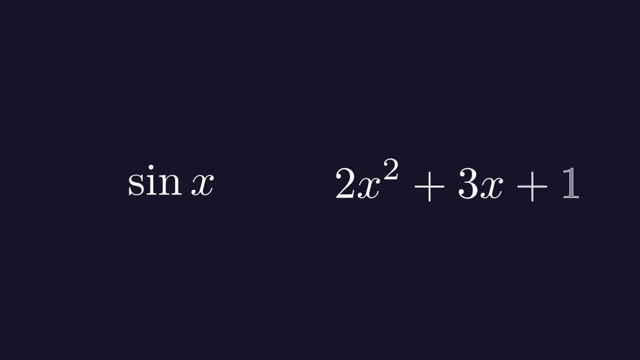 Brilliant will get 30% off Brilliant's annual premium service. Working with functions like sine and cosine is more complex than with polynomials. However, we can express these functions as infinite sums of powers of x, known as Taylor series. Let's assume that sine of x can't be expressed as an infinite polynomial. We can find the: 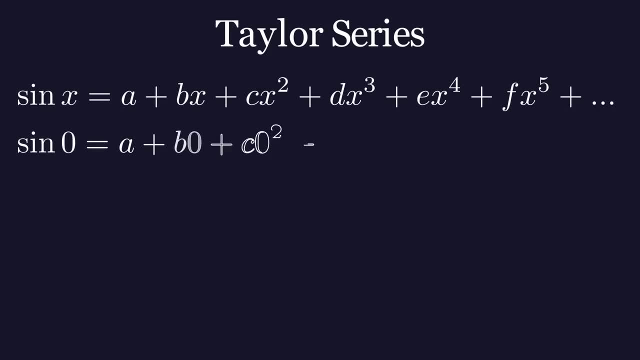 first term of this series. by plugging in zero for x, We get sine of zero on the left side, which is equal to zero. On the right side, we are left with only a, because the other terms becomes zero. So we get sine of zero on the left side, which is equal to zero. On the right side, we are left with only a, because the other terms become zero. 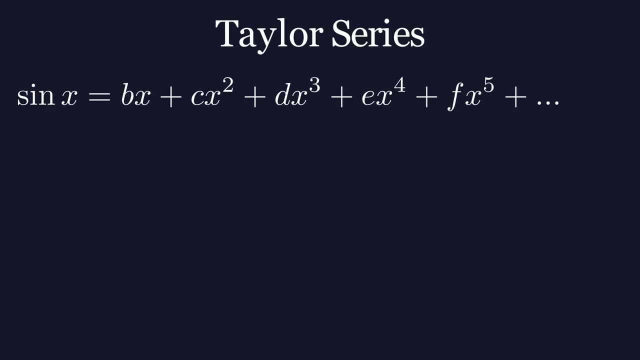 So a must be equal to 0.. Now we calculate the derivatives of both sides. Since the original functions are equal, their derivatives must also be equal. The derivative of sine of x is cosine of x. Using the constant sum and power rules, we can find the derivative of the right side. 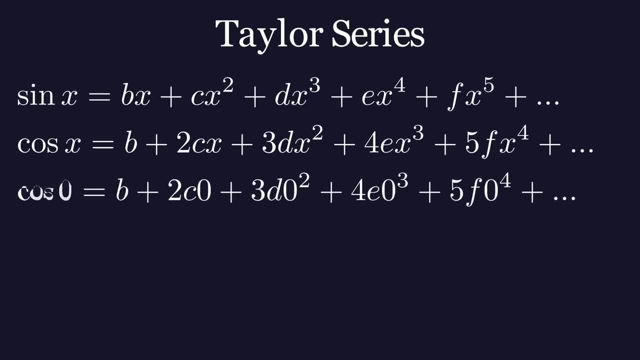 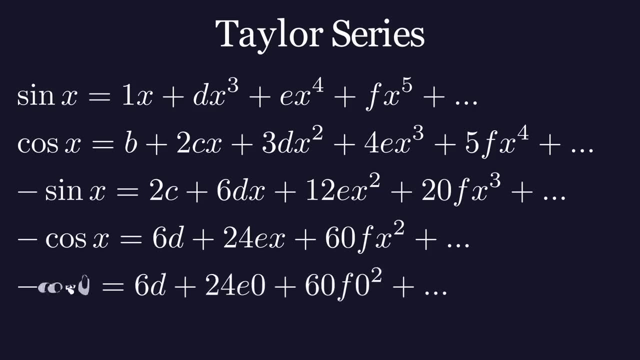 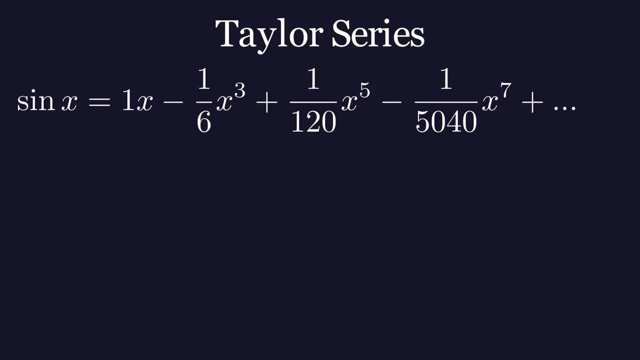 Now we set x to 0 again And we know that b is equal to 1.. Now we repeat this process again and again, And that gives us all coefficients. The denominators of the coefficients can be written as factorials of the odd numbers. 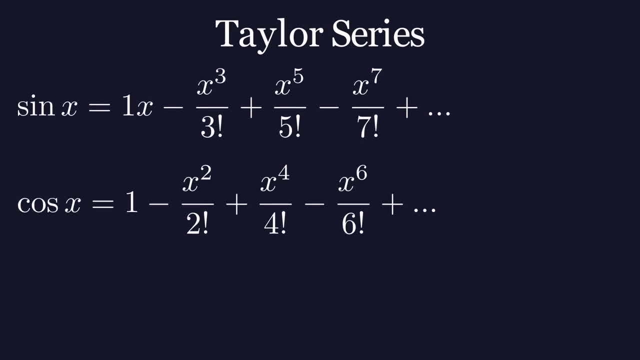 We can use the same method to find the Taylor series for cosine of x. To understand the concept of number e, let's look at exponential functions, For example f of x equal to 2 to the power of x. Since this isn't a polynomial, we have to use the definition to find its derivative. 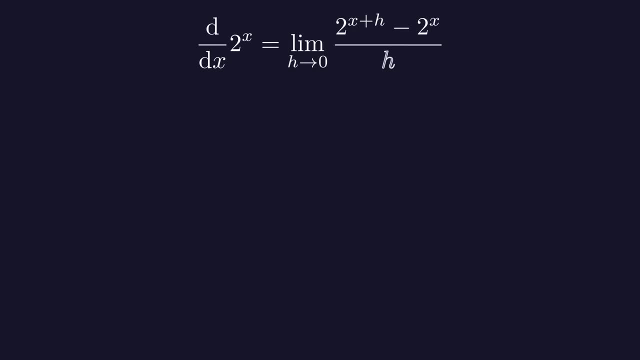 The derivative of this function is equal to the limit, as h approaches 0, of 2 to the power of x plus h, Minus 2 to the power of x divided by h. We can write 2 to the power of x plus h as 2 to the power of x times 2 to the power of. 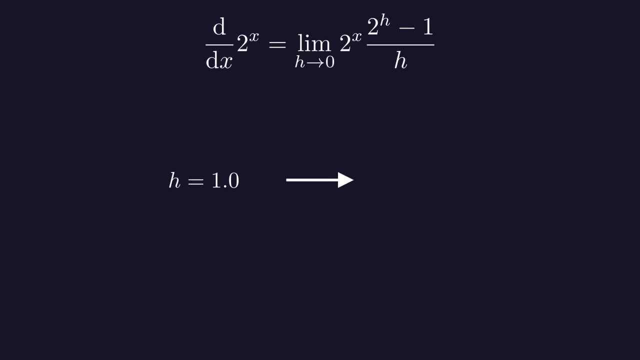 h. Now we can factor out 2 to the power of x. When we make h smaller and smaller, we find that this limit approaches a number around 0.69.. Let's do the same thing for 3 to the power of x. 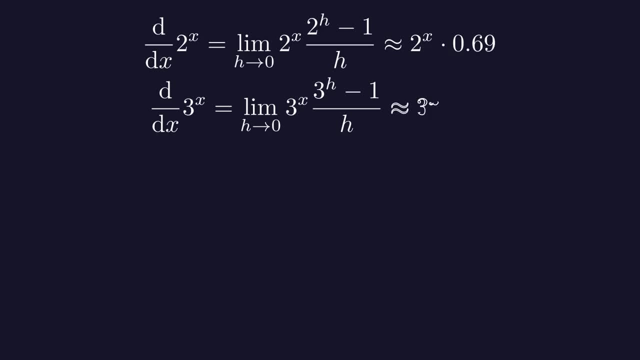 The derivative ends up being 3 to the power of x times around 1.1.. For 2 and a half to the power of x, the derivative is 2.5 to the power of x, The derivative is 2 to the power of x times around 1.1.. 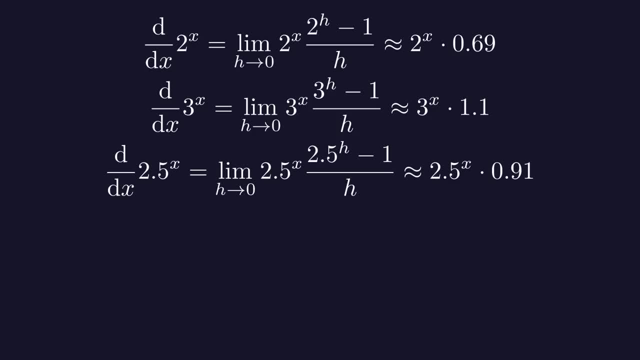 Now imagine we find a special number for which this part is equal to 1.. Let's call this number e. It means that the derivative of e to the power of x is equal to e to the power of x times 1.. So this function is its own derivative. 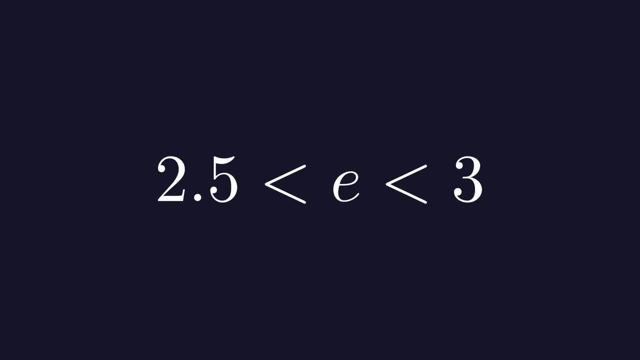 Now we only know that e is bigger than 2.5 and smaller than 3.. There are many ways to calculate the value of e, but first let's find a Taylor series for the function e to the power of x. We will use this function to calculate the value of e. 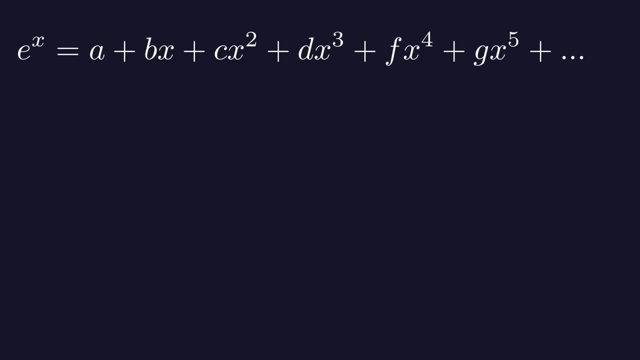 We will use the same method as we used to find the Taylor series for sine of x and cosine of x. We start by setting x to 0. This shows that the first coefficient is equal to 1.. Next we take the derivatives of both sides of the equation. 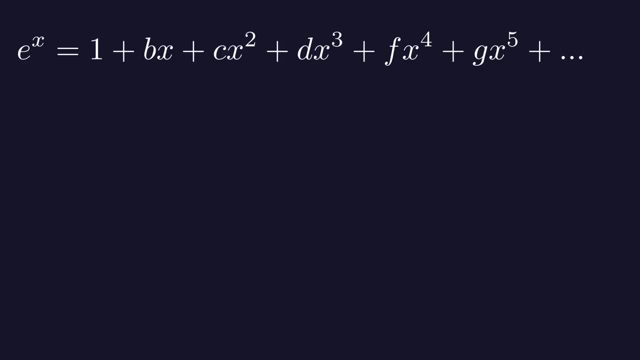 The left side, the derivative of e to the power of x is straightforward, because e to the power of x is its own derivative. For the right side, we use the constant sum and power rules. Then we set x to 0 again and we find that b is equal to 1.. 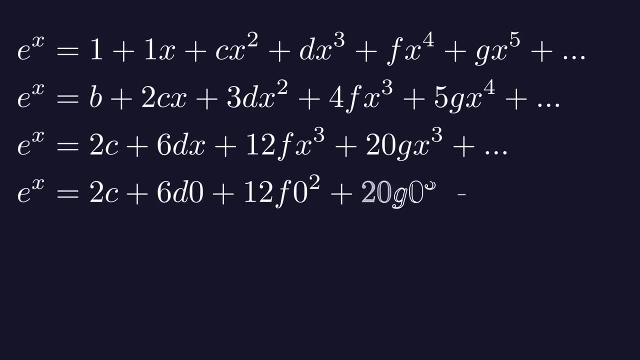 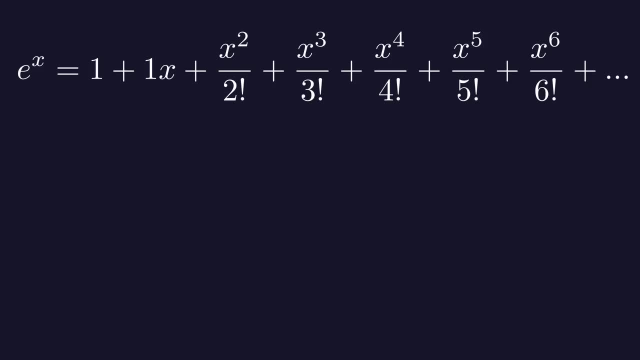 We repeat this process multiple times. This gives us the Taylor series for e to the power of x. To find the value of e itself, we can plug in 1 for x in the Taylor series and sum the terms. After summing the first seven terms of this series, we find that e is approximately equal.